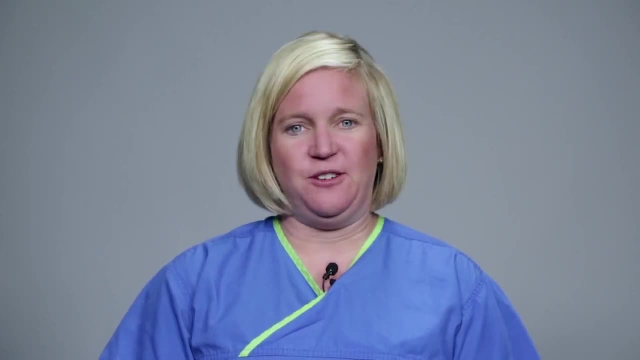 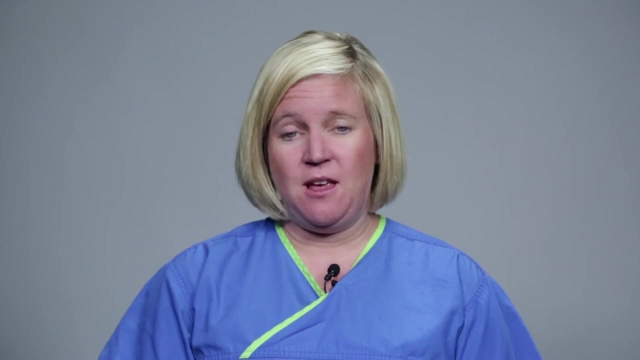 job is to take care of children that come into the hospital that have a burn injury. I teach these kids and their families how to care for the injury by helping them change the bandages. Another part of my job is to teach others on what a burn injury is and ways to keep children and 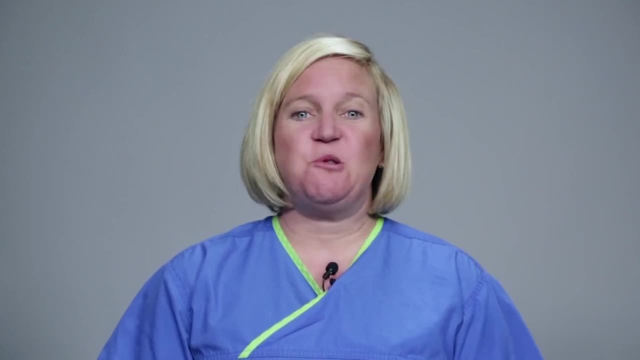 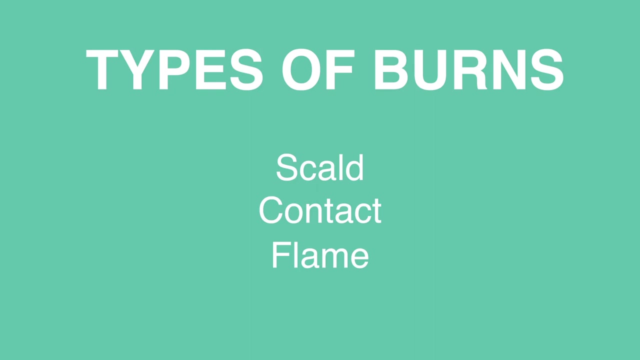 their families safe from these burn injuries. Let's do a quick overview of the types of burns. There's a scald, a contact and a flame burn. The most common injuries seen in the Children's Hospital include scald and contact burns. Scald burns occur most commonly in the kitchen. 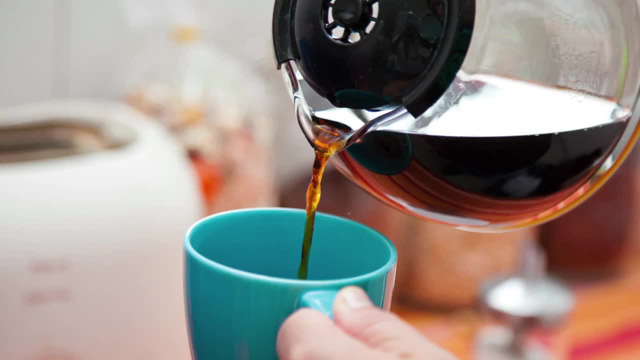 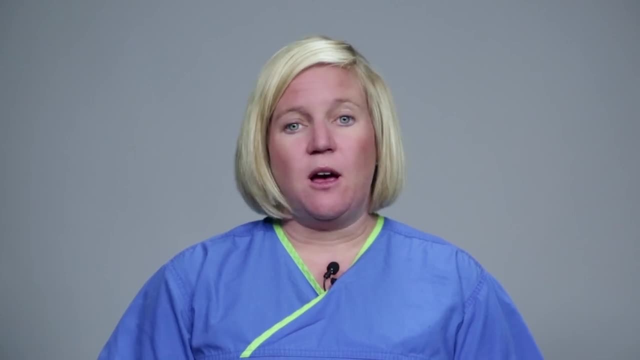 Hot liquids such as soup, coffee or boiling water are dangerous and you should never handle these by yourself. Always have an adult do this. Contact burns can be just as dangerous. These occur when you accidentally touch something that is hot enough to burn you. Some examples: 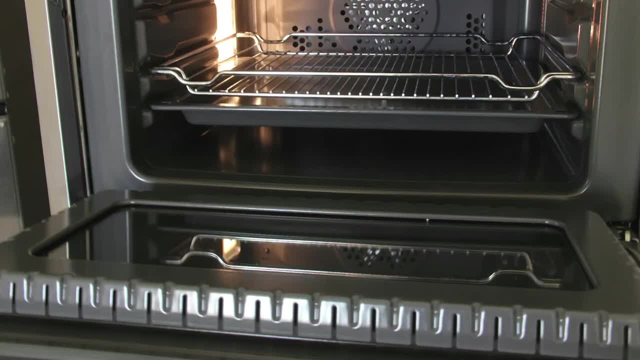 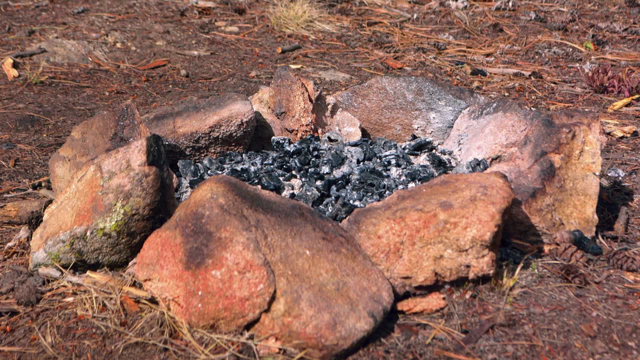 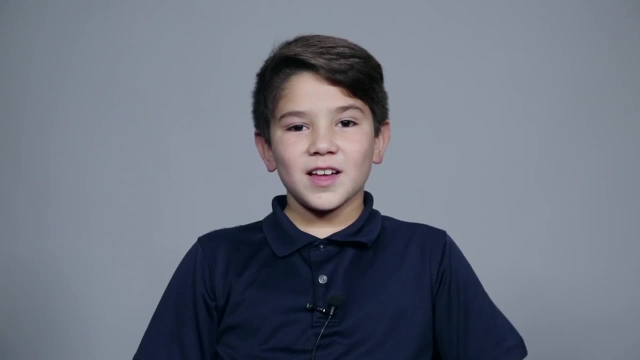 include grills, stove, oven doors, curling irons, fireplace or other hot items such as hot leaves or campfire ashes. What are the most common burns? Raise your hand if you like to help cook dinner or help out in the kitchen. 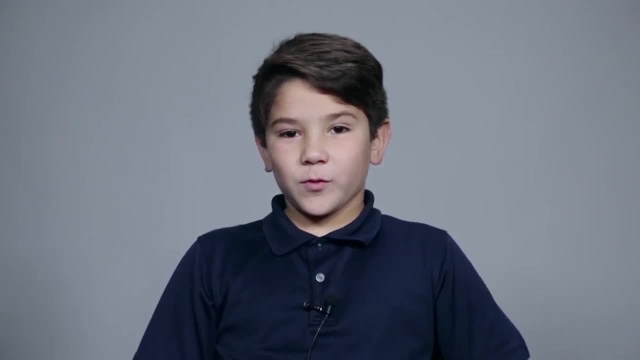 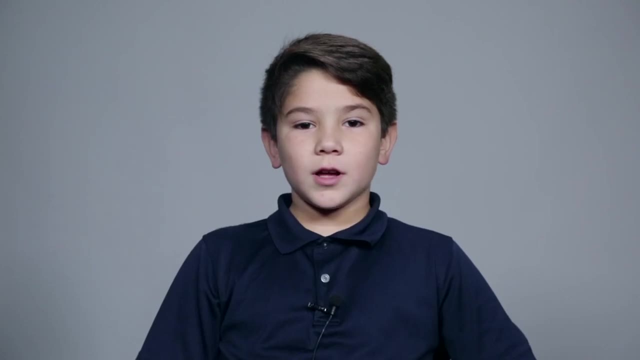 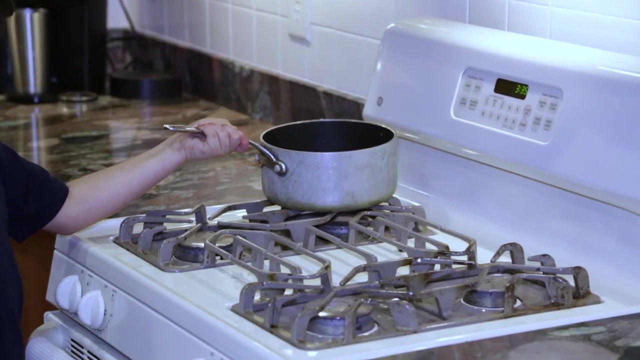 I see lots of you like to help out. That's great. These prevention tips are for you, then Listen and follow closely. We are going to walk through the house and make sure to use safety first. Have your parents use the back burners when cooking. Turn the pot handles away from the 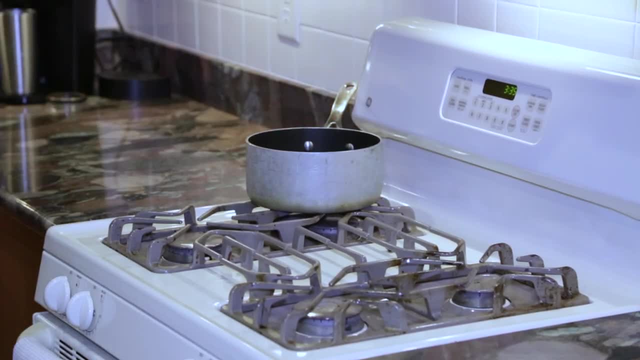 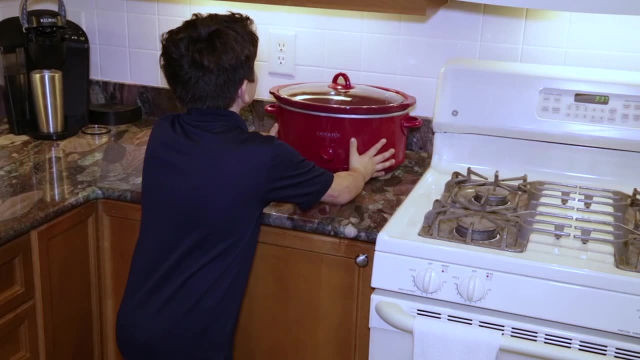 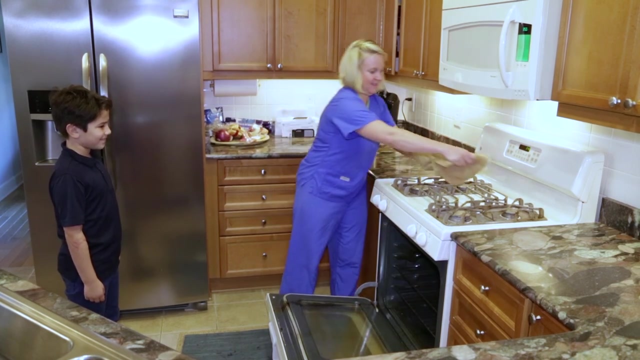 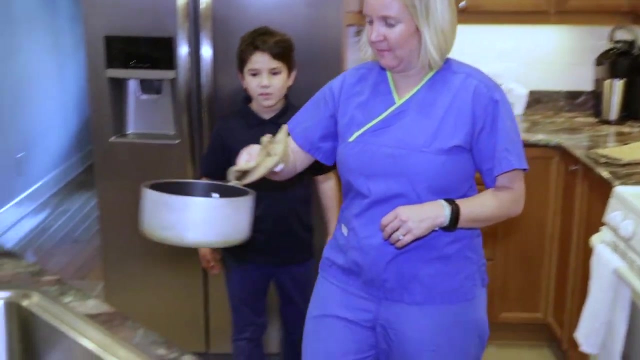 stove's edge. This prevents overturned pots. Make sure you have pots and pans containing hot foods or liquids. Make sure all appliance cords are kept coiled and away from the counter edges. Use mitt or pot holders when moving hot food from ovens, microwave ovens or stove tops. 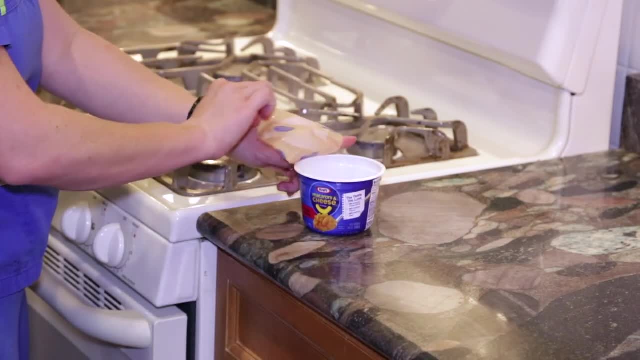 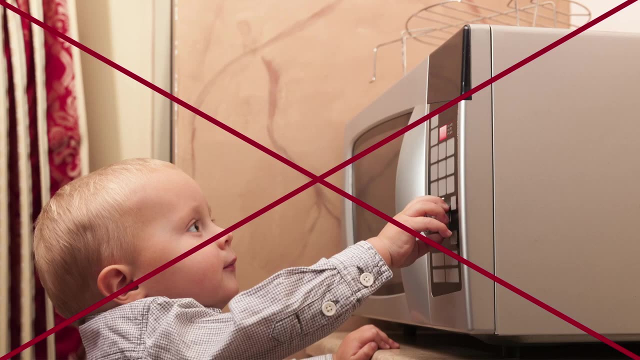 Open heated food containers slowly away from your face so the steam doesn't burn your face. Do not use microwave without help of an adult, because these items can be just as hot as if they were cooked on stove top. Do not hold a child while cooking, drinking or carrying hot foods and liquids.